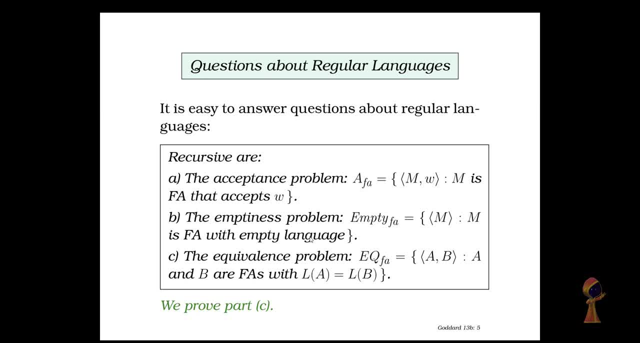 called decidable questions. The first one is something called the acceptance problem. So recursive languages are the acceptance problem. where A finite automata is the equal to M, W, M is a FA, or finite automaton that accepts W. 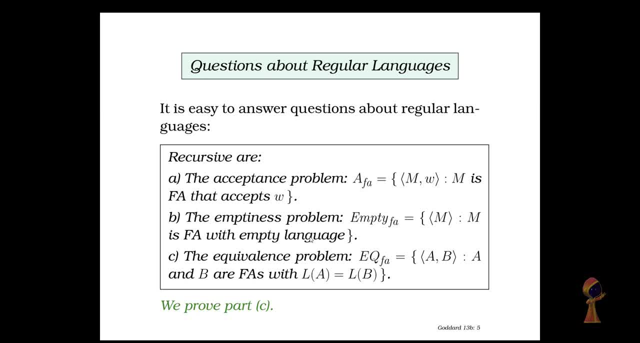 The emptiness problem- empty FA- where M is a finite automaton with empty language. The equivalence problem- EQFA- where A and B are finite automaton, with the condition that language of A is equal to language of B. Thank you. 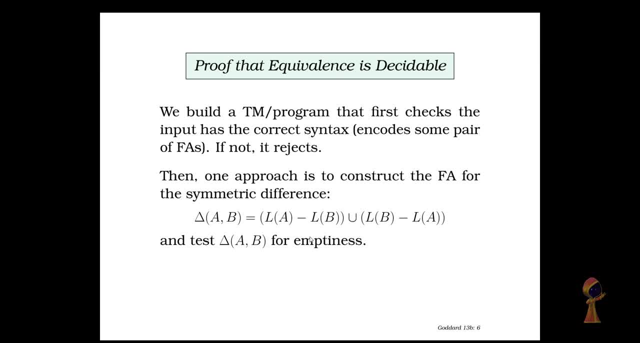 Thank you. In terms of proof, how do we do this? We can do a proof by construction. So we develop a build, or develop or build a Turing machine which first checks what is the input. Is the input in the correct syntax? If it's not in the correct syntax, then we cannot do the faulting. So we can do the first task, make the first test and test that Music playing: ploy, ploy, ploy, plow, plow, plow poun, plow plow peo, plow plow pepoo. we can do the proof If we use a conc struggle like that. we don't have the following: plow pew poo. width, trahh, int. peuvent we plow pew And we can it devices déjà plow in-put. canvgam hylrin가나 수. if there is an input enjoyed and not in the correct syntax. 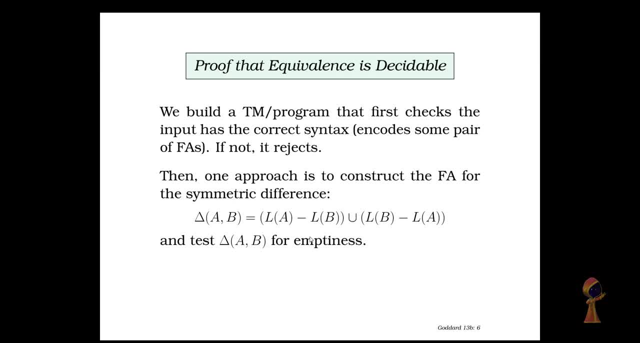 syntax, it's going to reject it, otherwise it will move to the main task and if you notice, this is very similar to how we check. we develop algorithm. so let's say, if we want to check password in a program, we're going to first see if the 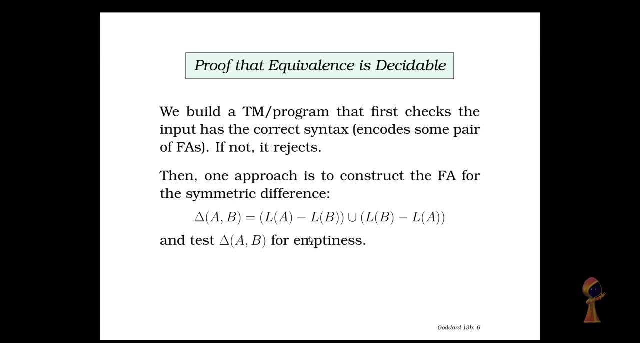 syntax is correct, and then we: if it is correct, then we'll allow the password to be saved, and next time if the user comes in and give the same password, then we check if it matches, and so on. so in Part C, with asking to check if two finite 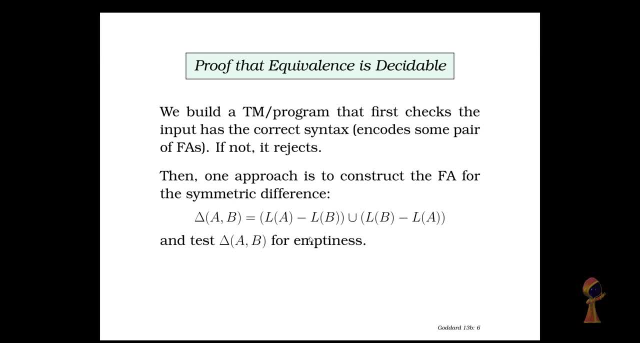 automata accept the same same language. so how do we do this thing? we can construct the finite automata for the following reasons: we can construct the finite automata for the following reasons: language, which is called Delta, a, B. Delta means the symmetric difference and in a. 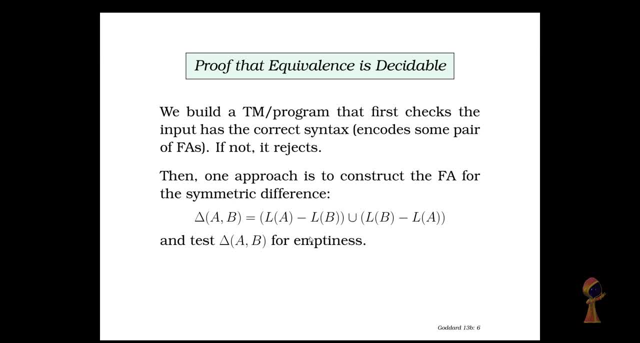 symmetric difference. it is equivalent to length, the difference of the two languages both ways. so we are essentially looking at language of a minus language of B. this is one set union, language of B minus language of a. so it's symmetric. so both sides are considered whatever is. 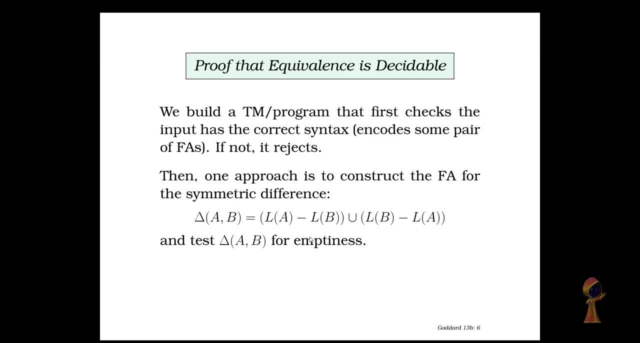 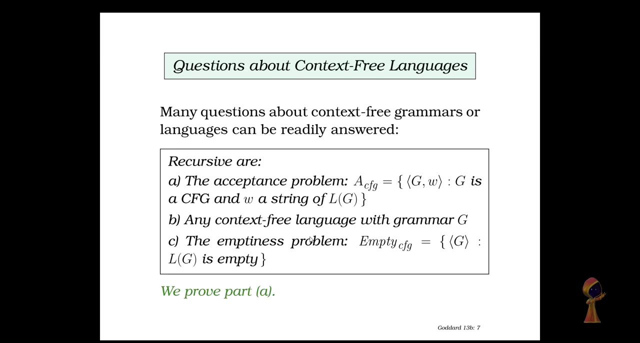 not there and check to see if it is empty. so one sweetest this emptiness, we can use the facts based on the tomorrow. so language of a minus land with a P is equal to language of a complement, union language of being and old complement. and if you want to talk for 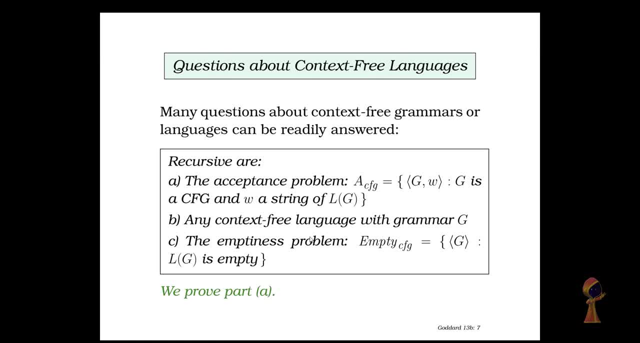 context-free languages we can say there are recursive in the sense of first the acceptance problem. so a context-free grammar is recursive, which is the acceptance problem, so it is accepting. when G is a CFT context-free grammar and w is a string of language of that grammar, then any context free language. 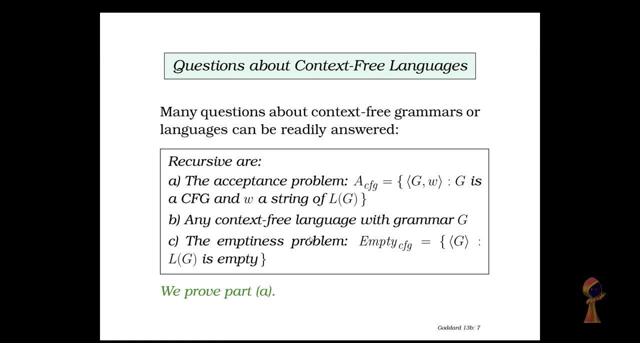 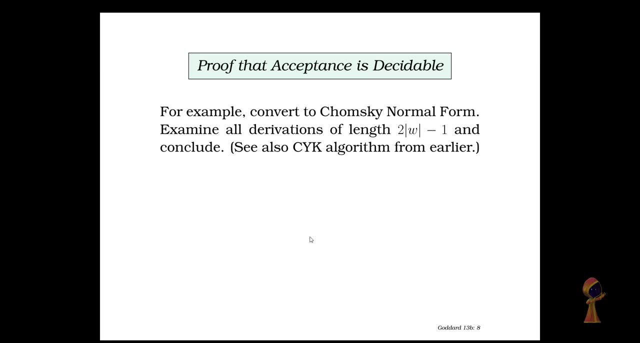 with grammar G itself, its recursive. then the emptiness problem. so empty, context-free grammar is a grammar where language is empty. so if want to prove one of these, let's say part a: we can convert the grammar which is a context-free grammar and we can convert the grammar which is a. 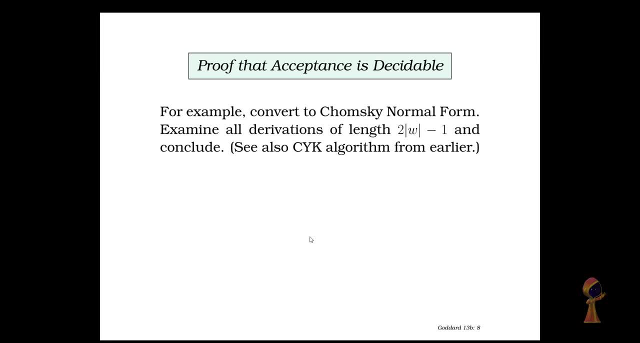 to CNF, which is Chomsky normal form, and then check all the derivations of length to W or length of W minus 1, and then conclude, so, for example, write G on the tape, pass the program in the first step, and so on. now one thing which is 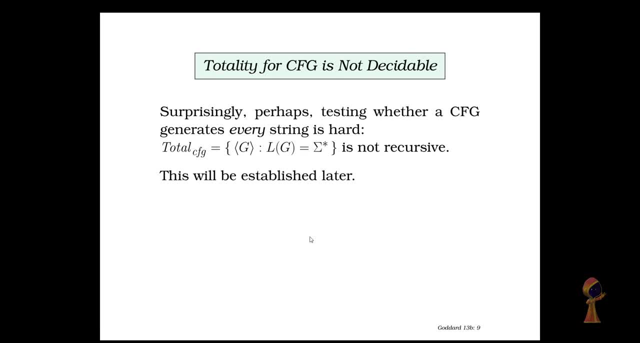 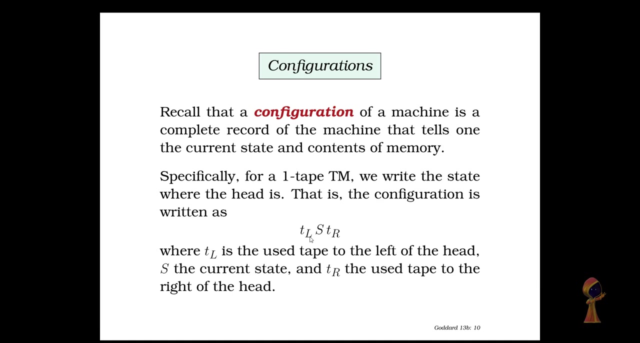 surprising is that the totality for a context-free grammar is not decidable. what does that mean? it mean testing whether a CFG generates every possible string. this is a very hard problem, so total CFG is not recursive. this results is something which we will establish later on. now let's talk about the concept of 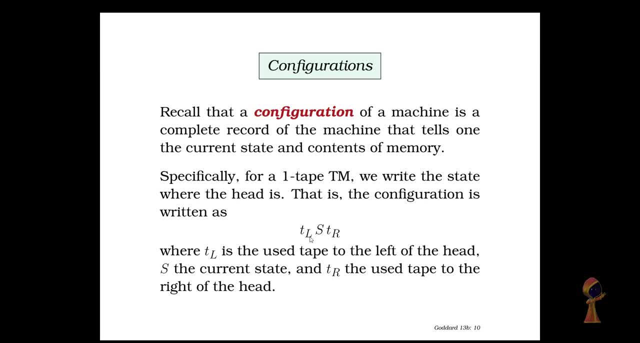 configurations. now, configuration tells the complete record of the machine. so it says: this is the current state, this is the content of the memory. so if we've got a one tape Turing machine, we write the state so such that the tape on the left side is on the left and then s is the state and tape on the 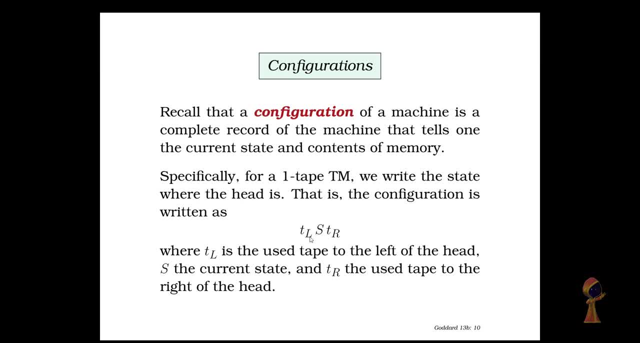 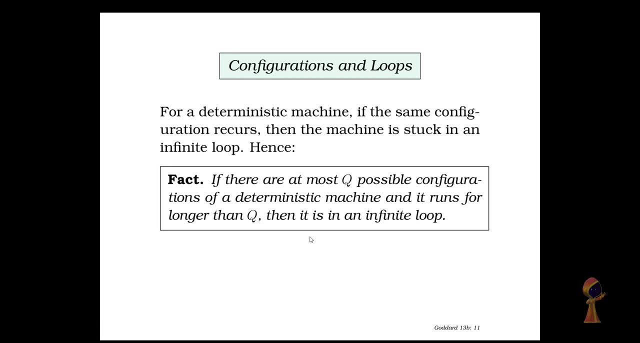 right is written on the right now, remember, TL is the use tape to the left now, if we talk about configurations, remember there is a possibility of a loop. what does that mean? so if the machine is deterministic and the same type of configuration occurs again, that means we are in an infinite loop. so if there at most, Q possible, 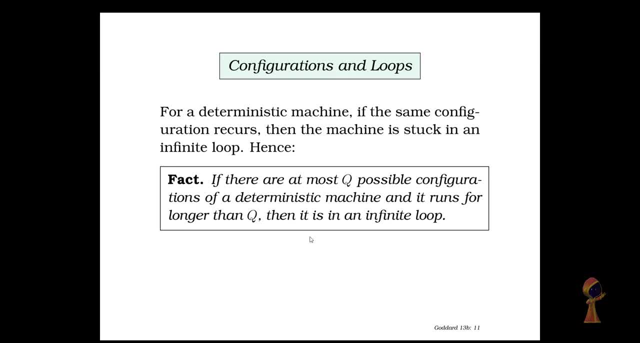 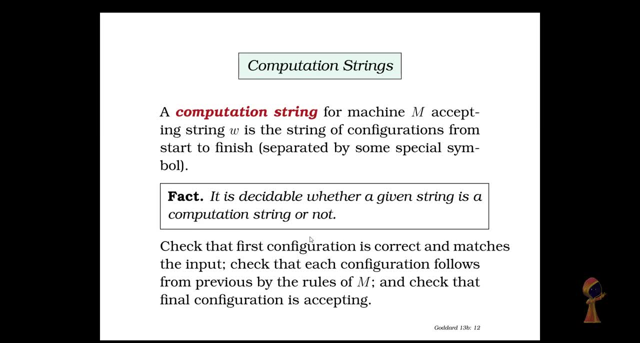 configuration, And if it runs for longer than q, then that means it's an infinite loop. Another concept to look at is that of a computation string. A computation string for a machine M accepting a string W is a set of configurations. It's a string of configuration from start of finish. 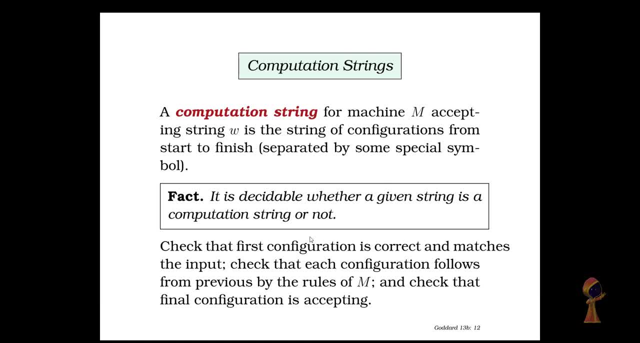 And between these configurations we can have some special symbol. So the fact is it is decidable whether a given string is a computation string or not, How We can start with the first one And see if it matches the input and then keep going with every step. and if it matches, 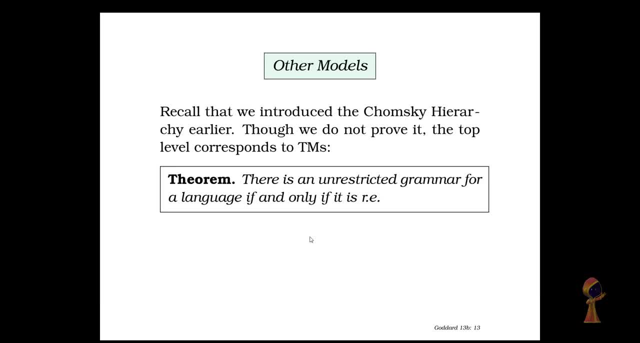 till the end, then it is decidable. so so this is a decidable problem. now there are other models of computation as well, so these include an unrestricted grammar and other grammars. so now the top level of that Chomsky hierarchy corresponds to Turing machine. there is a theorem. we say that there is an. 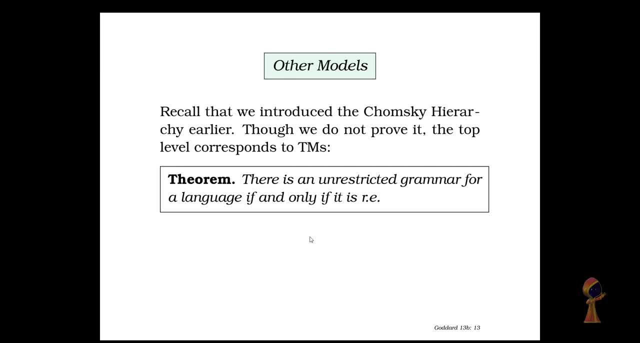 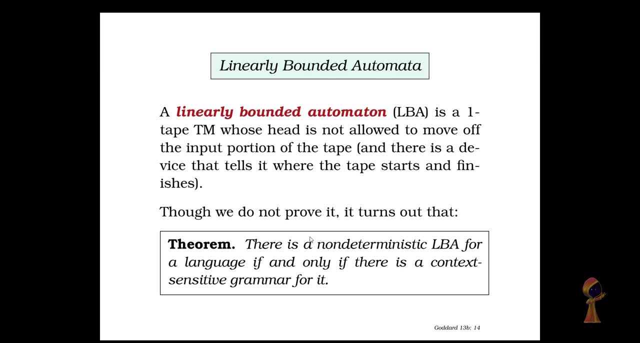 unrestricted grammar for a language if, and only if, it is recursively enumerable. there are other models of computation, for example an LBA, which is a linearly bounded automaton. LBA is a one-tape Turing machine where the head is not allowed to move off the input portion of 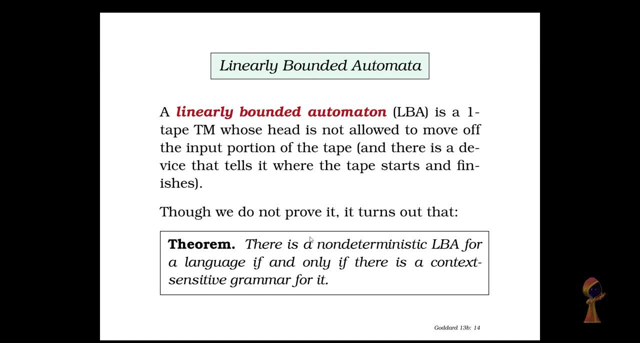 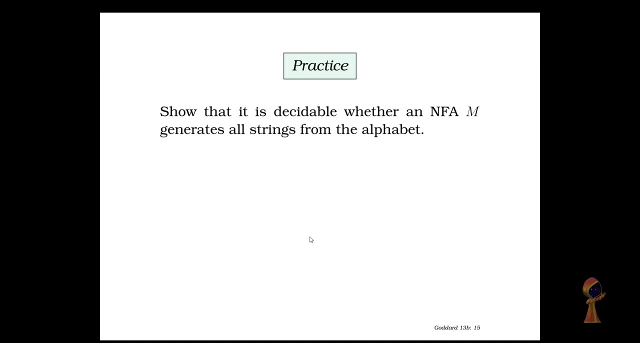 the machine. so there's also a device which tells us whether, where the tape starts and finishes. so there is a theorem, there is a, a, a non-deterministic LBA for a language if, and only if, there is a context sensitive grammar for it. so to practice, you can show that it is decidable. 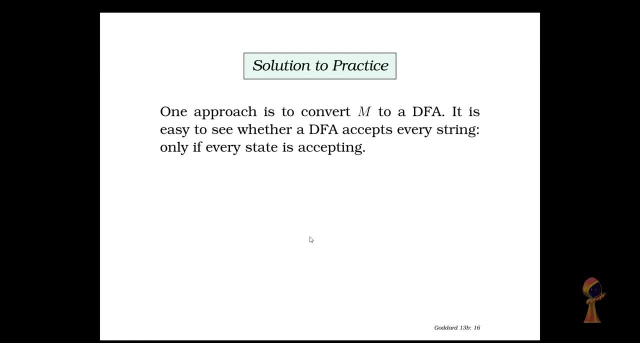 whether an NFA M generates all strings from the alphabet, and one solution to that is convert the M to a DFA because it was an NFA, so convert it to a DFA, and then you can see whether or not the DFA accepts everything only if every state is. 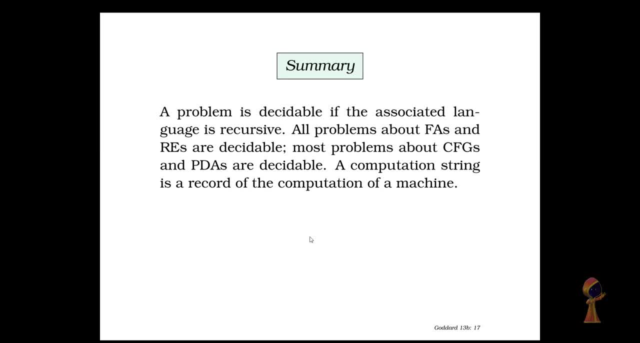 accepting. so it will only accept it if every state is also accepting. so in summary, a problem is decidable if the associated language is recursive. all problems about finite automaton order and regular languages, regular expressions are decidable and most problems about CFG context not to take effect if every state is accept. so it will only accept if every state is. tän sẽ không ACend if the associated language is recursive. all problems about finite automaton languages, regular expressions are decide double and most problems about cfg context. we 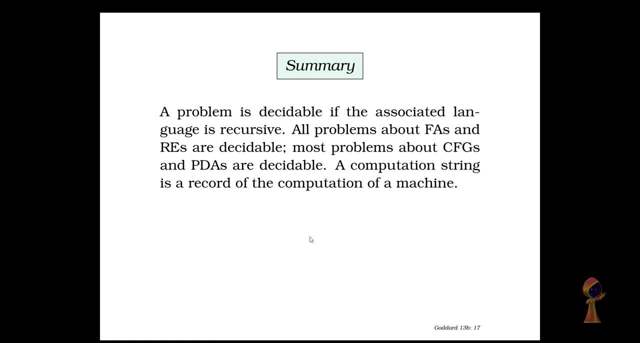 grammars and push-down automata's are also decidable, most but not all. so our computation string is a record of the computation of a machine.